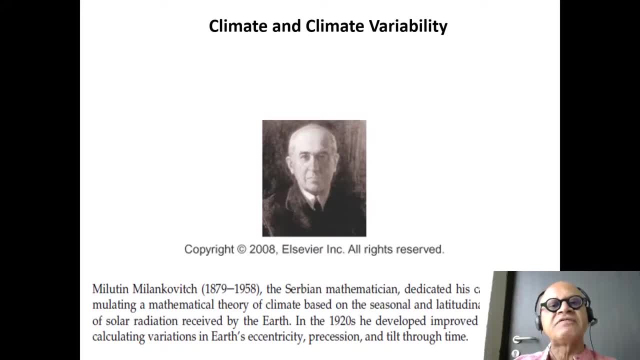 feedbacks because, as we will see, it's the internal feedbacks that take the solar radiation coming in and produce a very rich spectrum of timescales. Okay, There are some big names: Militin- Milankovic always comes up- was the first guy to mathematically formulate the changes in Earth's orbital parameters, as we will see later, The glacial, deglacial cycles, or 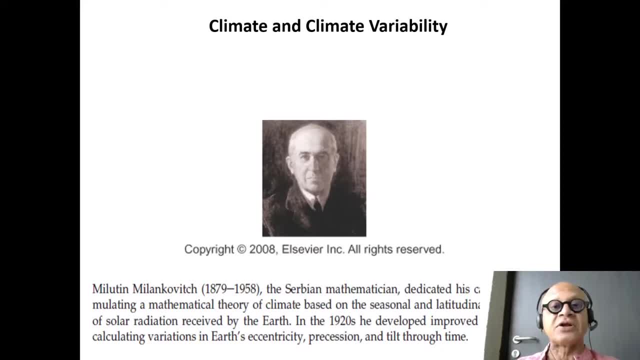 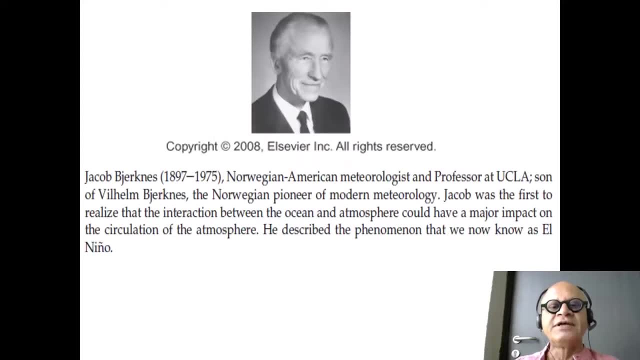 ice ages, like ice age cycles, are referred to as Milankovic cycle. There was James Crowell before him, much before him, who also had similar ideas. Jakob Birkness is famous for his work on El Nino related feedbacks. He was the son of the famous Wilhelm Birkness which we had talked about in the previous chapter. 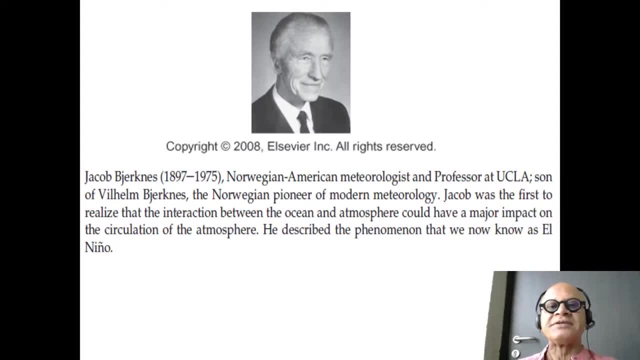 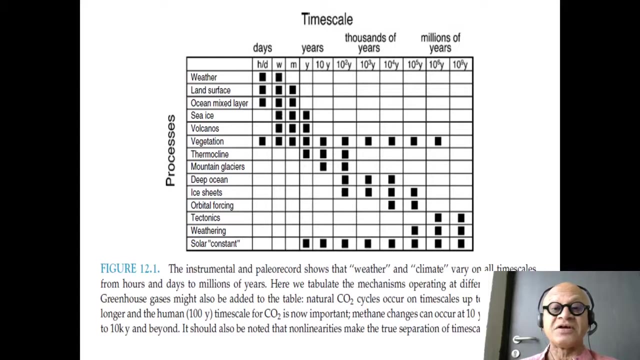 And we will see what Jakob Birkness did. that makes him a very important person at the short timescales of interannual variability, specifically El Nino. So there are this whole range of timescales of climate variability, going from weathers which occur on hours and days, land surface, going from days to months, ocean mixed layers and so on. 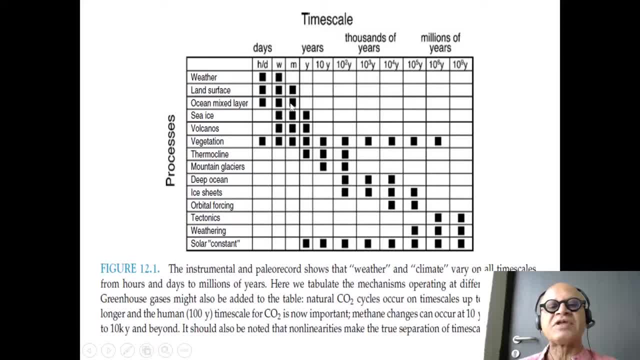 Just the surface layer is along the same timelines: Sea ice begins to get into years, Volcanoes, which are very episodic, vegetation you can see, begins to go into million year timescale because it has feedbacks and it moves slowly, It has memory and so on and so forth. 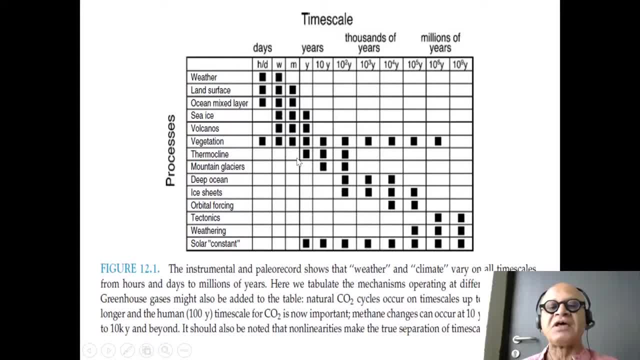 There are many ways to say it, but we will see what we mean. We split into surface layer, thermocline and depotion, which produce very different timescales. Mountain glaciers, depotion, ice sheets, orbital forcing, that's the militant Milankovitch cycles. 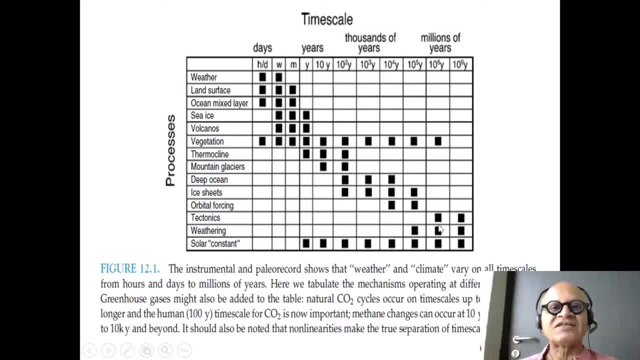 Tectonics, we will see how continental drift has had big impacts on climate as well. Weathering is the geologic timescale, Control on carbon dioxide and, of course, solar constant, Which happens on monthly to yearly and decadal and all the way to billion year timescales. 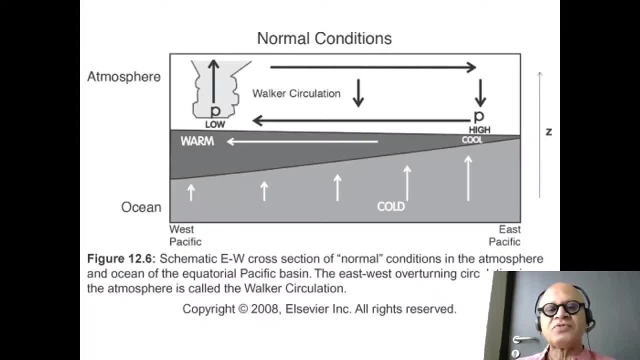 Okay, we will learn about El Nino, which is the most dominant variability from year to year timescale. so-called inter-annual variability is related to the things we have already looked at in terms of upwelling in the east, cold temperatures, piling up of water in the west, warm temperatures, sea surface temperature and so on. 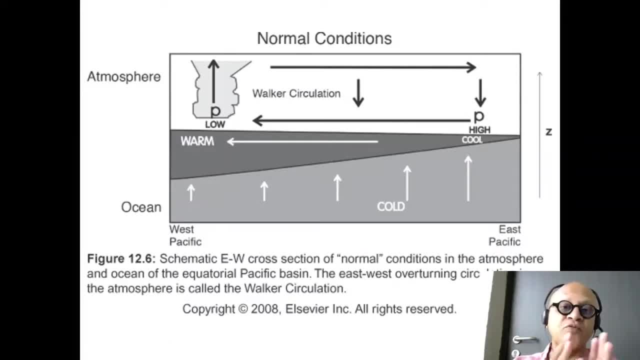 Temperature gradients because Coriolis is low. you also have wind response, pressure response and we have, of course, deep convection here And the local zonal circulation which we didn't talk a lot about. We always talked about zonal, mean meridional cells, but there is a very important zonal cell that becomes very important. 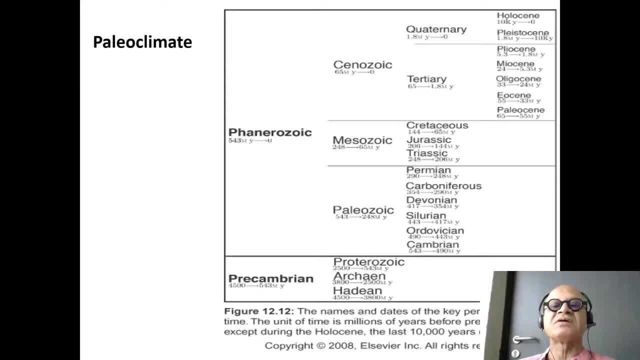 We'll touch on paleoclimate at various timescales. There are these periods we will talk about pre-campus Cambrian. Cambrian is around 540 million years ago, when there was a huge explosion of new species. Before that, you had Hadean. actually, that's Hades hell in Greek. 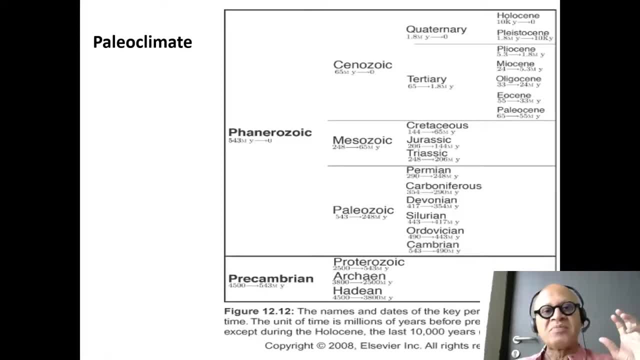 And Hadean is when there was bombardment. primordial soup- not any evidence of life as far as we know, Archean comes from Arches, which means the beginning, where we get the earliest evidence of biotic elements in the rocks and so on. 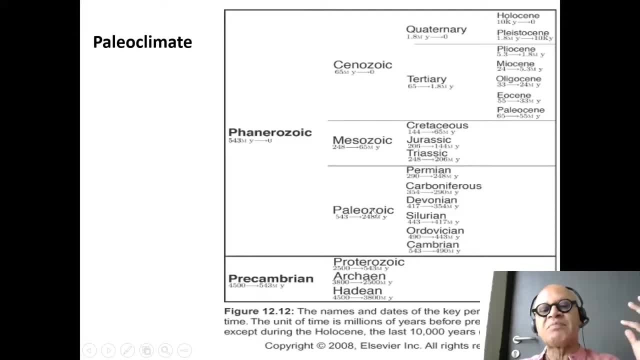 And then you get Proterozoic, which means early life, then you get Paleozoic and then Mesozoic, Cenozoic. we are now, Typically, we keep saying Holocene, but the new geologic era has been defined, beginning at the Industrial Revolution. 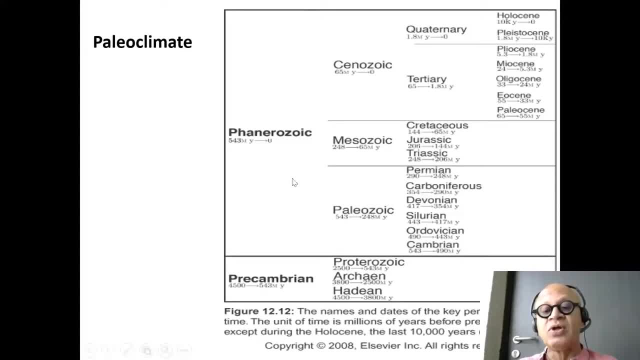 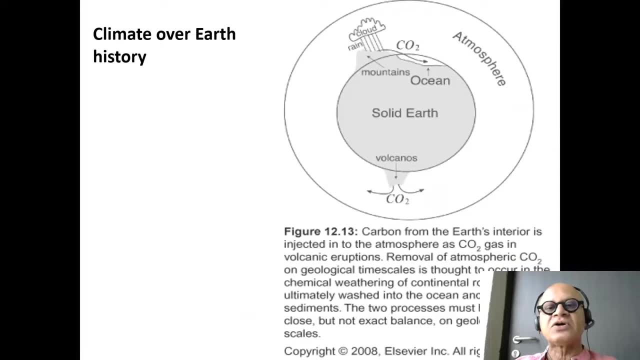 And it's now called Anthropocene. so we will talk about what's happening in the Anthropocene. So we will talk about what's happening in the Anthropocene, Okay, so let's see. the climate, or Earth's history, Obviously has feedbacks from volcanic forcing, solar forcing, the feedbacks between solid Earth on long timescales, continental drifts and so on.